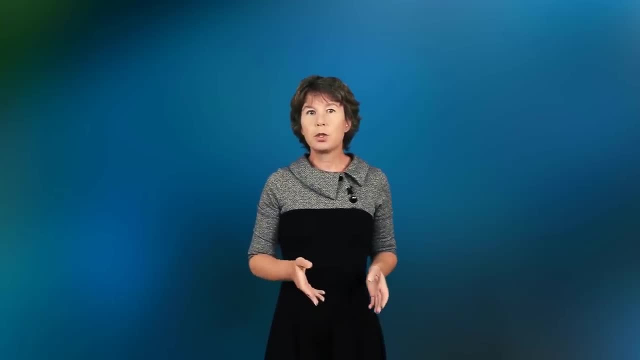 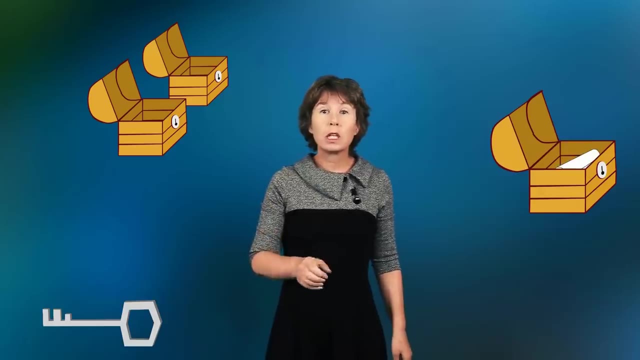 You can think of this as if the website you are buying from gives you not a key, but an empty treasure chest that locks when you close it. You take the chest, put in your credit card number, close it, and now the only person who 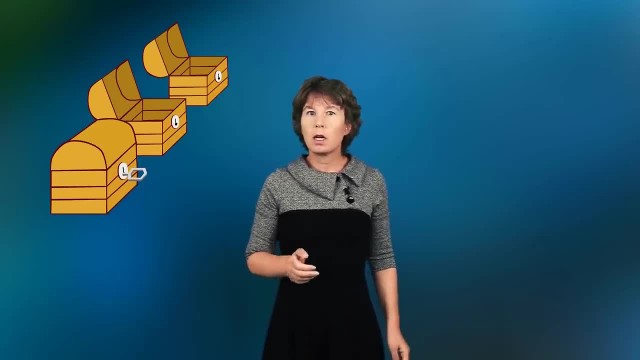 can open, it is the one who knows how to unlock it. So your message is safe to send. In practice, that treasure chest is locked by a mathematical problem that is easy to pose but really hard to solve. There are various mathematical problems that can and that are. 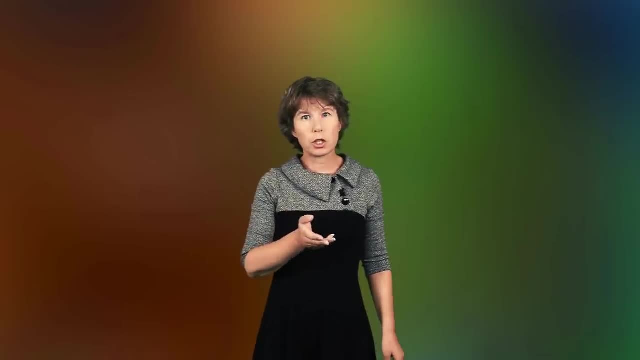 being used in cryptographic protocols for locking the treasure chest. The best known one is the factorization of a large number of keys. The key is to lock the treasure chest. This method is used by the algorithm known as RSA, after its inventors, Rivers, Charmier and Edelman. 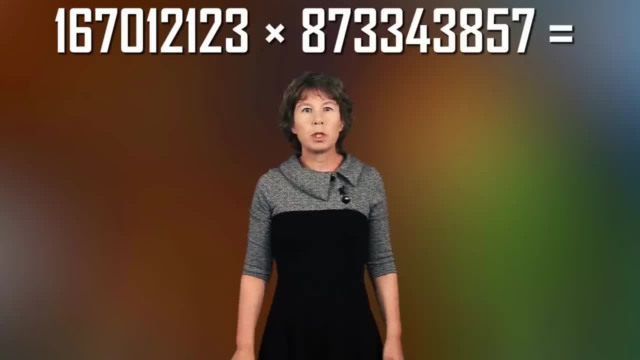 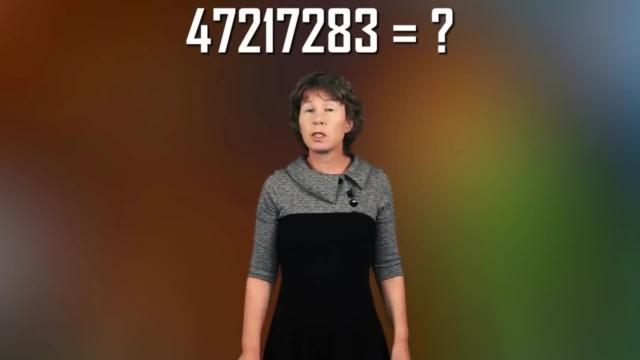 The idea behind RSA is that if you have two large prime numbers, it is easy to multiply them, But if you only have the product of the two primes, then it is very difficult to find out what its prime factors are. For RSA, the public key, the one that locks the treasure chest, is a number. 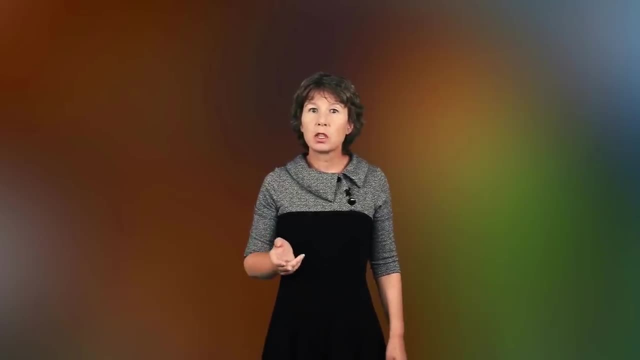 that is derived from the product of the primes but does not contain the prime factors themselves. You can therefore use the public key to encode a message, but to decode it you need the prime factors, which only the recipient of your message has, for example the retailer. 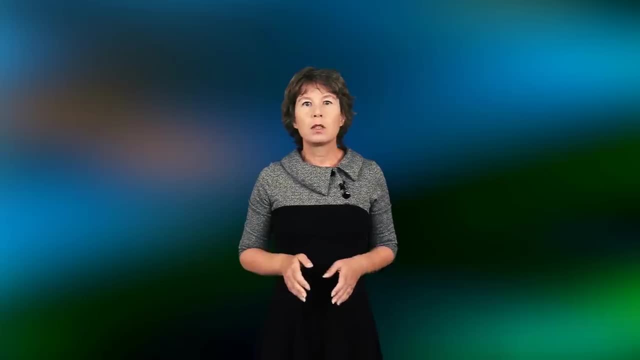 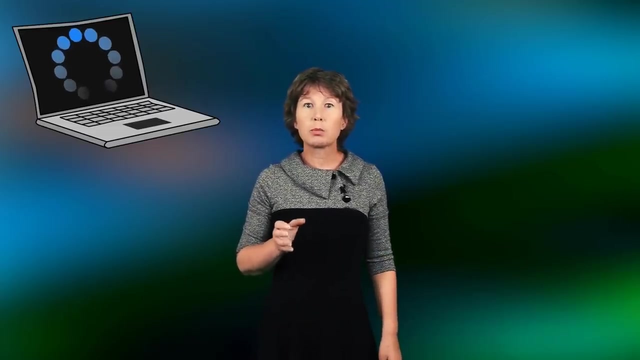 to whom you are sending your credit card information. Now, this public key can be broken in principle, because we do know algorithms to decompose numbers into their prime factors, But for large numbers, these algorithms take very, very long to give you a result, even on the world's presently most powerful computers. 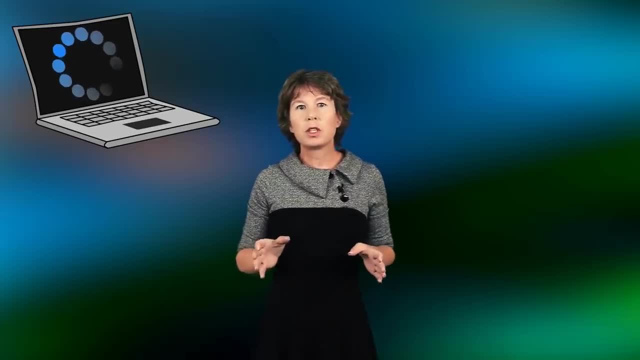 So maybe that key you are using can be broken, given a hundred thousand years of computation time. But really, who cares? For all practical purposes, these keys are safe. But here's the thing: Whether or not someone can break one of these public keys depends. 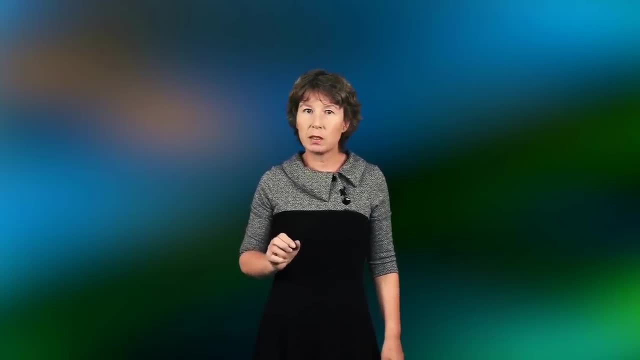 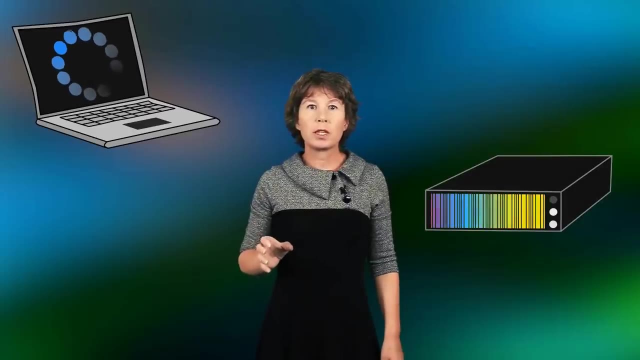 on how quickly they can solve the mathematical problem behind it, And quantum computers can vastly speed up computation. You can see the problem: Quantum computers can break cryptographic protocols such as RSA, And that is a big security risk. I explained in a previous video what quantum computers 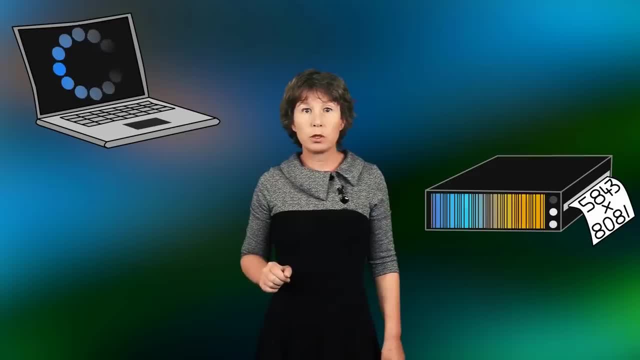 are and what to expect from them. so check this out if you want to know more. But just how quantum computers work doesn't matter so much here. It only matters that you know. if you had a powerful quantum computer, it could break some public key cryptosystems. 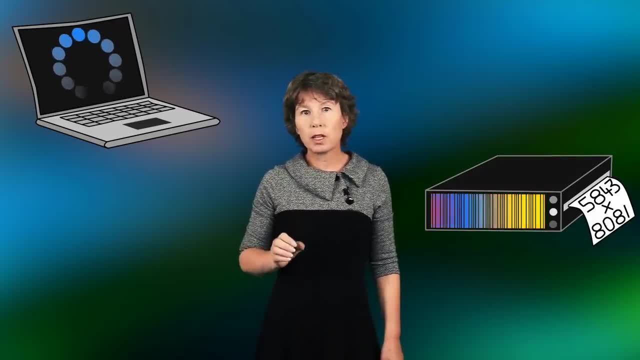 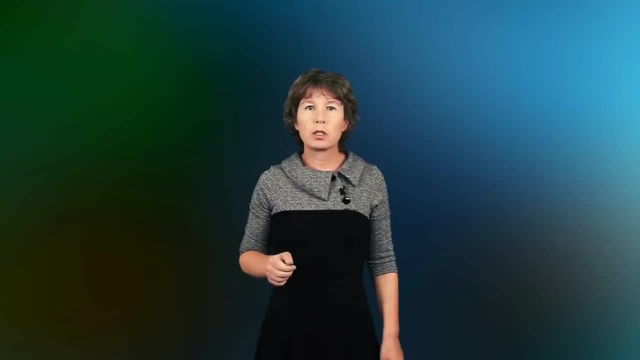 that are currently widely being used, and it could do that quickly. This is a problem that can only affect your credit card number, but really everything from trade to national security. Now we are nowhere near having a quantum computer that could actually do such a computation, But the risk that one could be built in the next decades is high. 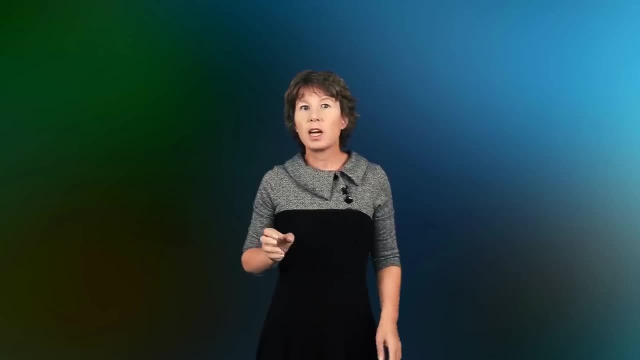 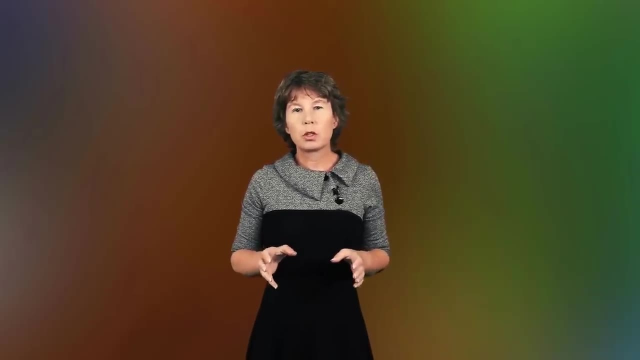 enough so that computer scientists and physicists have thought of ways to make public key cryptography more secure. They have come up with various cryptographic protocols that cannot be broken by quantum computers. This is possible by using protocols which rely on mathematical problems for which a quantum computer does not bring 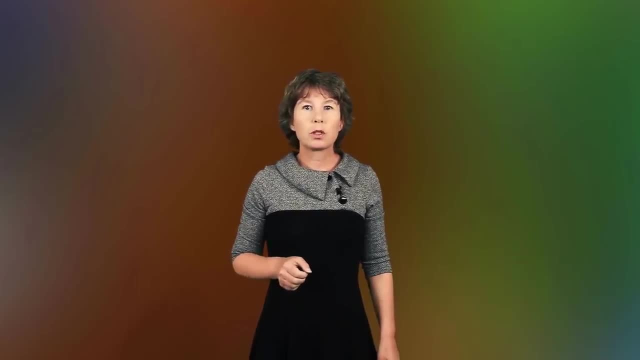 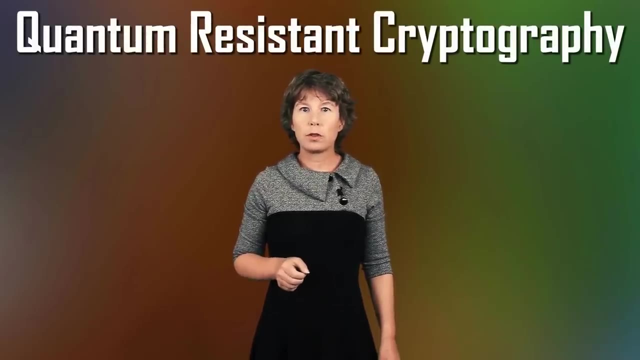 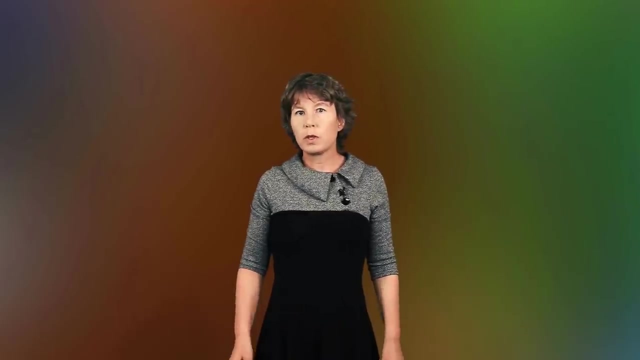 an advantage. This cryptography, which is safe from quantum computers, is called post-quantum cryptography, or sometimes quantum-resistant cryptography. Post-quantum cryptographic protocols do not themselves use quantum effects. They have the word quantum in their name merely to say that they cannot be broken, even with quantum. 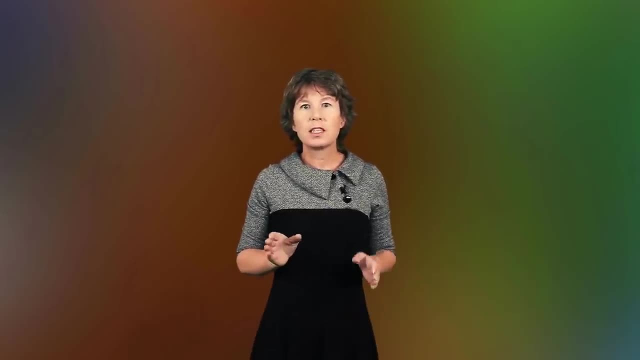 computers, At least according to present knowledge. This situation can change, because it's possible that in the future, someone will find a way to use a quantum computer to break a code currently considered unbreakable. However, at least at the moment, some cryptographic protocols exist for which no one knows how. 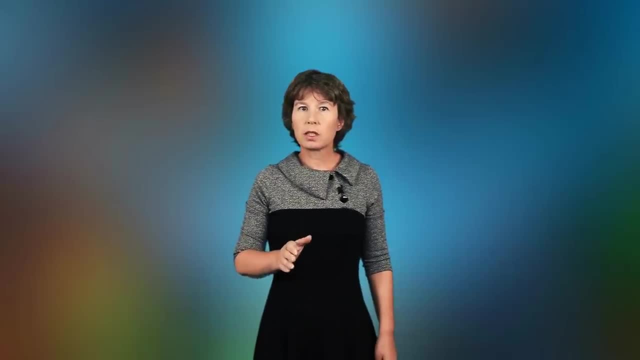 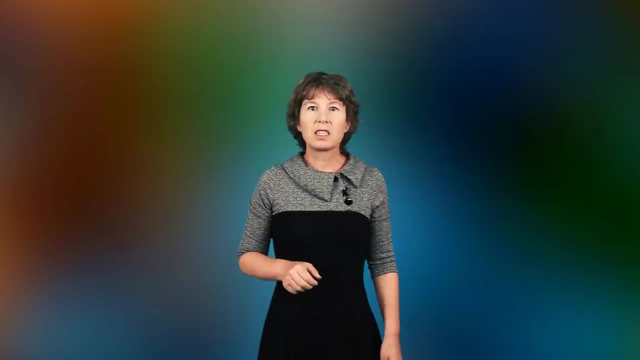 a quantum computer could break them. So computer scientists have ways to keep the internet safe, even if someone somewhere develops a powerful quantum computer. Indeed, most nations already have plans to switch to post-quantum cryptography In the coming decade, if not sooner. 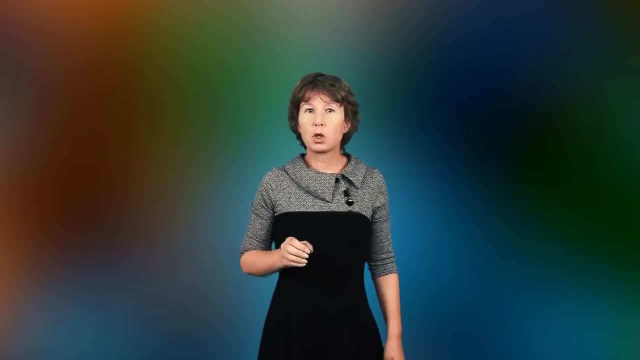 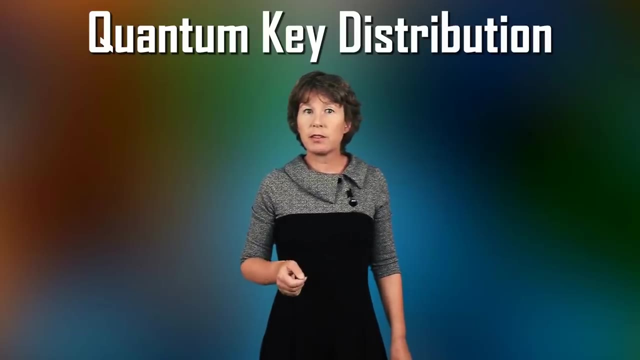 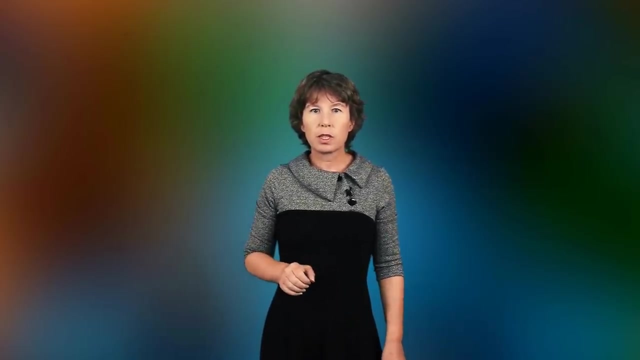 Let us then come to quantum cryptography and its application for quantum key distribution. Quantum key distribution is a method for two parties to securely share a key that they can then use to encode messages, And quantum physics is what helps keep the key safe. To explain how this works, I will again just use the simplest example, that's a protocol. 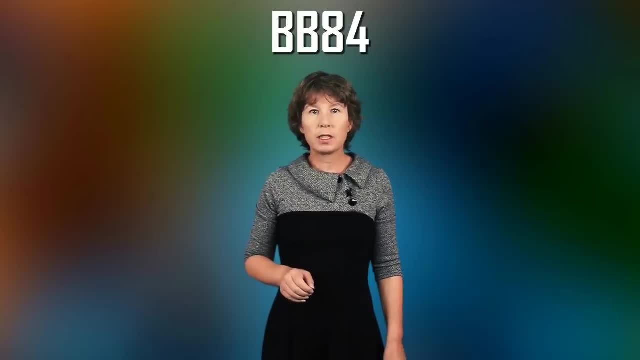 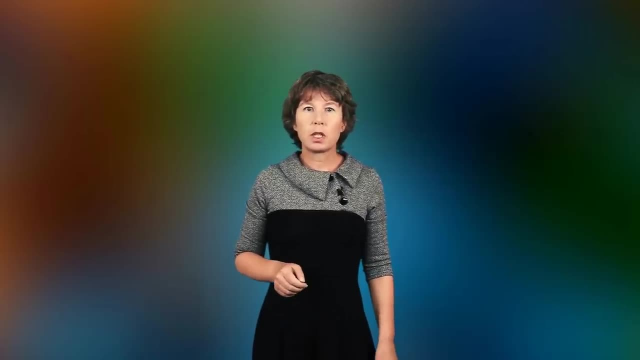 known as BB84, after the authors Bennett and Brassard and the year of publication. When physicists talk about information transfer, they like to give names to senders and receivers. Usually they are called Alice and Bob, so that's what I will call them too. Alice wants. 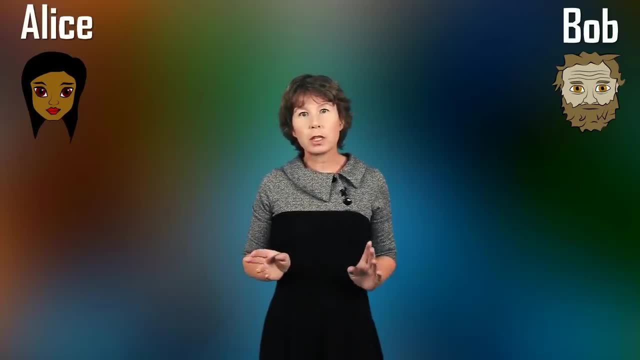 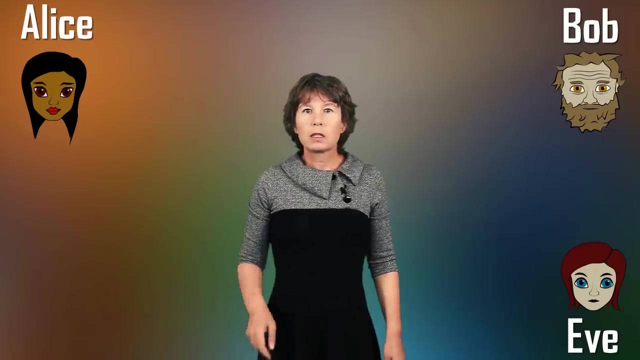 to send a secret key to Bob so they can have a little chat, but she does not want Bob's wife, Eve, to know what they are talking about. In the literature this third party is normally called Eve because she is eavesdropping. Hahaha, physics humor. So Alice creates a random sequence. 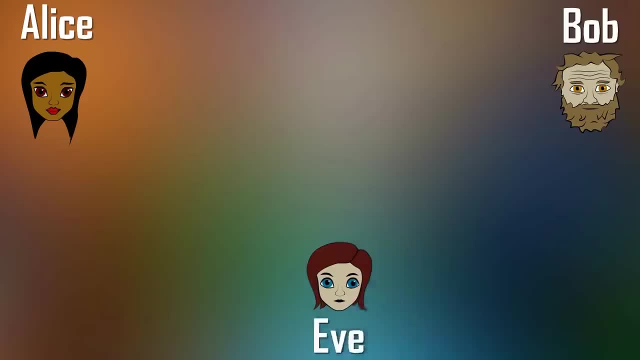 of particles that can have spin either up or down. She measures the spin of each particle and then sends it to Bob, who also measures the spin. Each time they measure spin up, they note down a zero, and each time they measure spin down, they note down a one. This way, 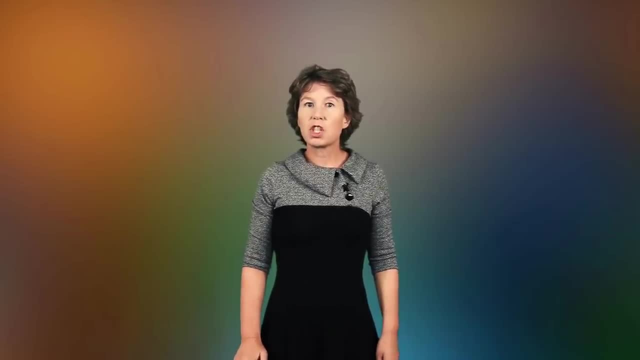 they get a randomly created shared sequence of bits which they can then use to encode messages. But this is no good. The problem is this key can easily be intercepted by Eve. She could catch the particle meant for Bob in M and send it to Bob with it. Bob and Eve will have to alternate between the same key. 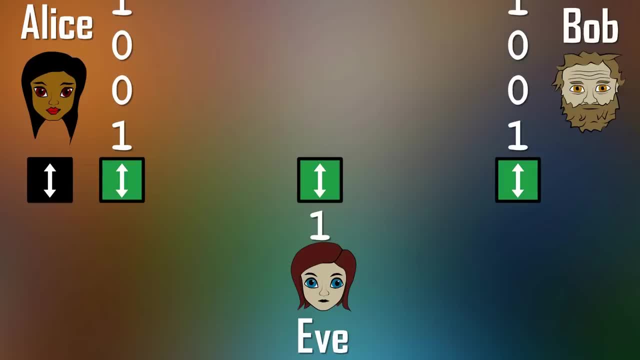 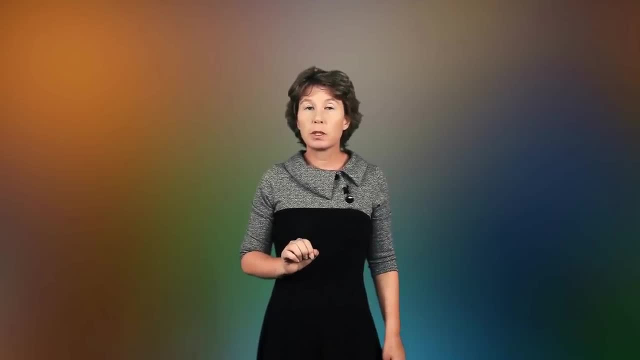 flight, measure it, note down the number and then pass it on to Bob. That's a recipe for disaster. So Alice picks up her physics textbooks and makes the sequence of particles that she sends to Bob more complicated. That the spin is up or down means Alice has to choose a direction along. 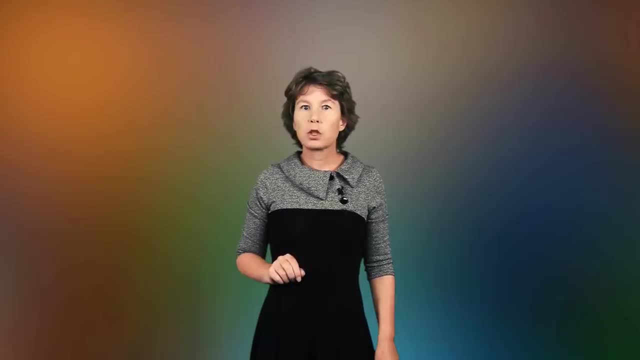 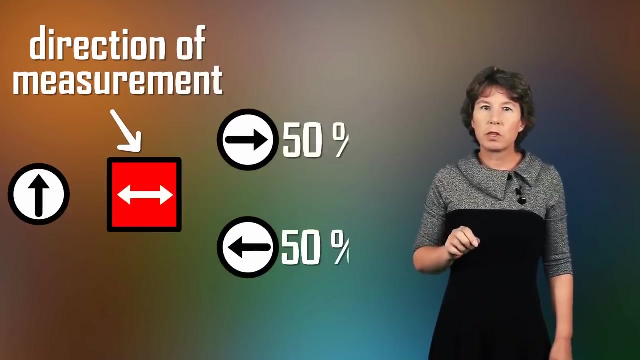 which to create the spin. Bob has to know this direction to make his measurement, because different directions of spins obey an uncertainty relation. It is here where quantum mechanics becomes important. If you measure the spin into one direction, then the measurement into a perpendicular direction is maximally uncertain For a binary variable like the spin. this just 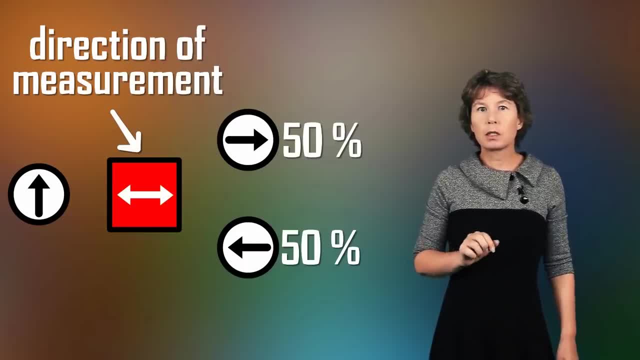 means the measurements in two orthogonal directions are uncorrelated. If Alice sends a particle that has spin up or down, but Bob mistakenly measures the spin in the vertical direction, he just gets left or right with fifty percent probability. Now what Alice does. 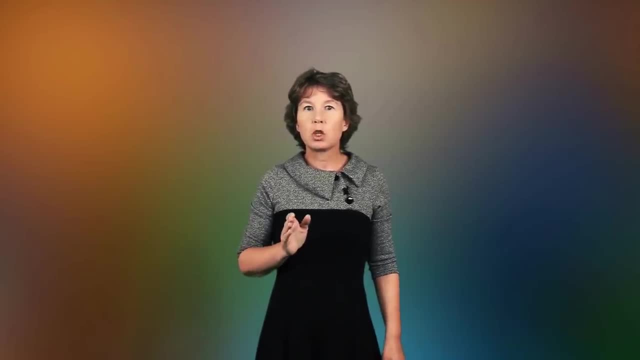 is to randomly choose whether the particle's spin goes in the up, down or left right direction, As before. she sends the particles to Bob but- and here is the important bit- does not tell him whether the particle was created in the up down or left right direction. 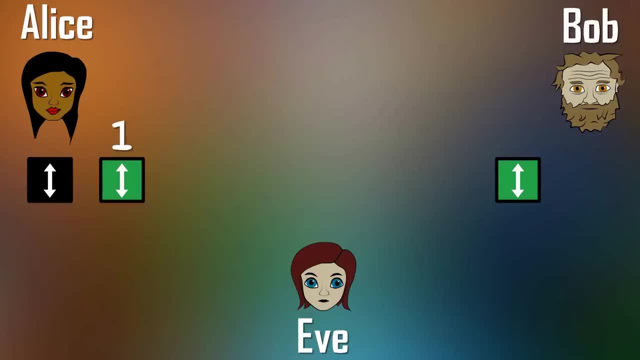 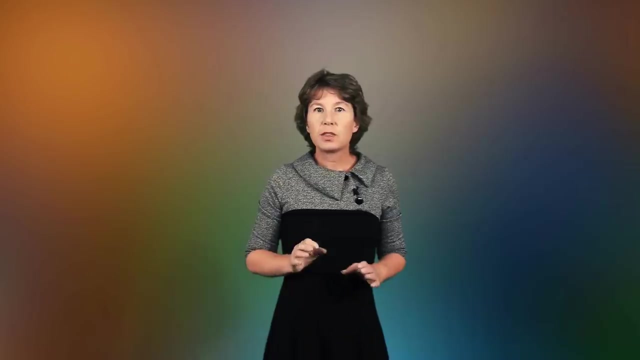 Since Bob does not know the direction, he randomly picks one for his measurement. If he happens to pick the same direction that Alice used to create the particle, then he gets, as previously, a perfectly correlated result. But if he picks the wrong one, then he gets a completely uncorrelated result. After they have done that, Alice sends. 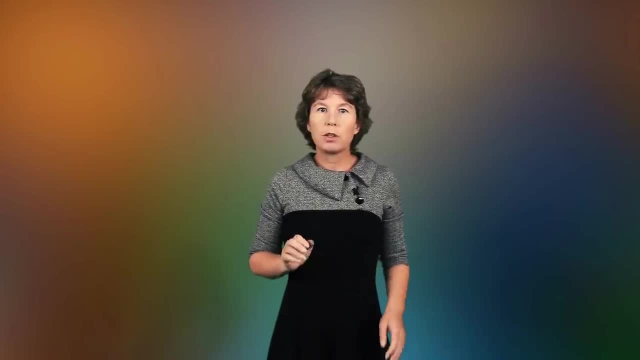 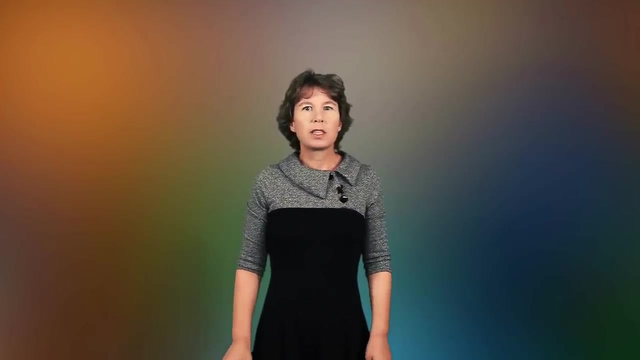 Bob information about which directions she used. For that she can use an unencrypted channel. Once Bob knows that, he discards the measurements where he picked the wrong setting. The remaining measurements are then correlated and that's the secret key. What happens now if Eve tries to intersect the key that Alice sends? 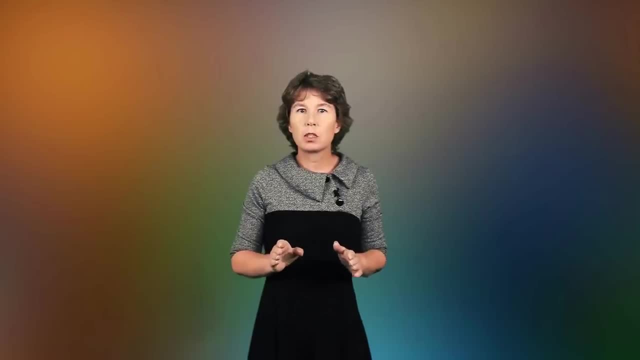 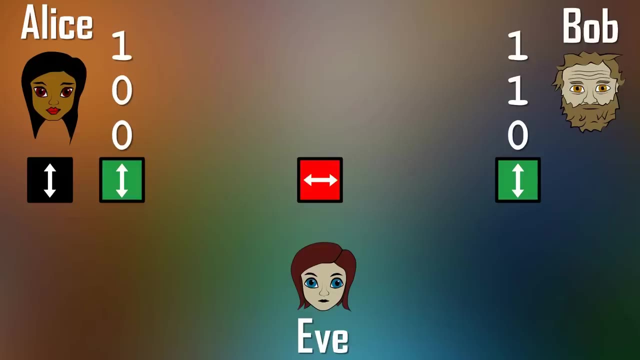 Here's the thing: She cannot do that without Bob and Alice noticing. That's because she does not know either which direction Alice used to create the particles. If Eve measures in the wrong direction, say left right instead of up down. 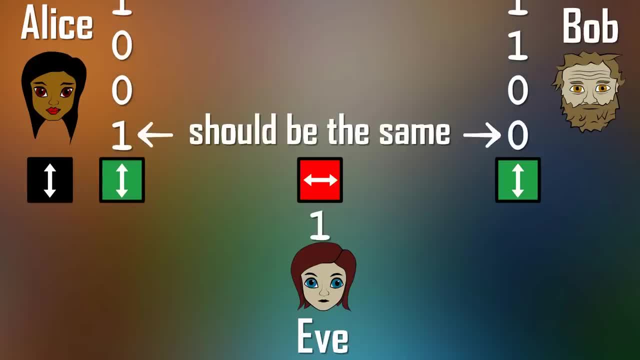 she changes the spin of the particle, but she has no way of knowing whether that happened or not. If she then passes on her measurement result to Bob- and it's a case where Bob did pick the correct setting- then his measurement result will no longer be correlated with Alice's. 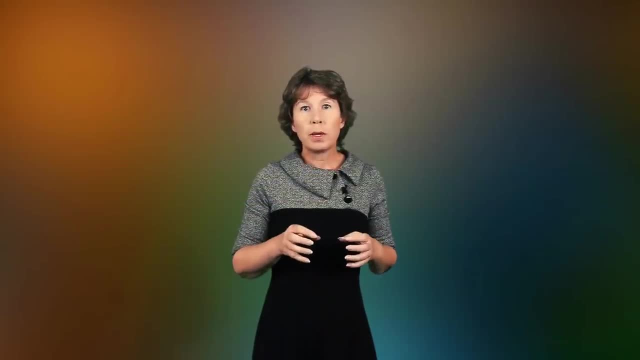 when it should be. So what Alice and Bob do is they compare some part of the sequence they have shared. Again, they can do that using an unencrypted channel and they can check whether their measurements were indeed correlated when they should have been. If that's not the case, they know someone tried to intercept the message. 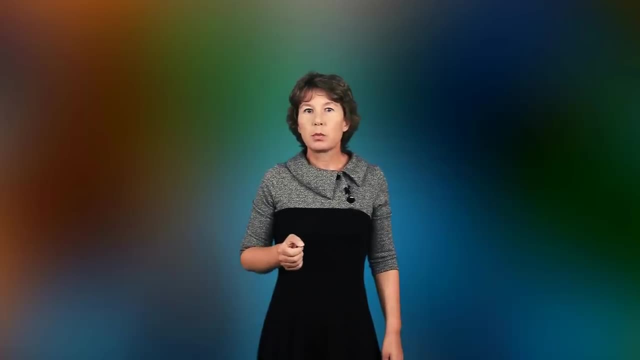 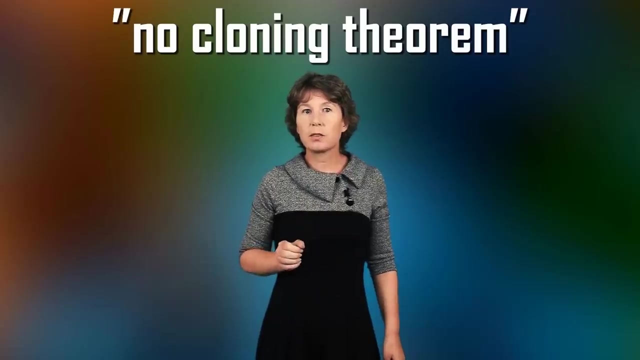 This is what makes the key safe. The deeper reason this works is that in quantum mechanics, it's impossible to copy an arbitrary state without destroying it. This is known as the no-cloning theorem, and this is ultimately why Eve cannot listen in without Bob and Alice finding out. 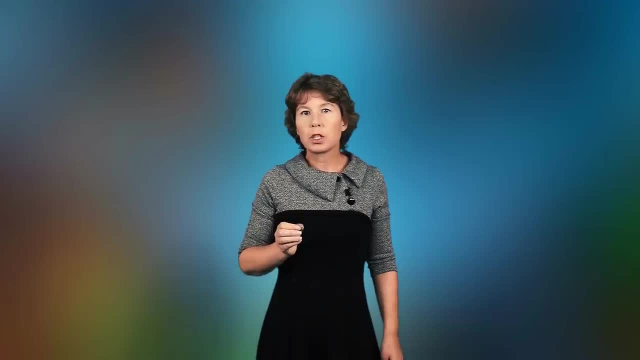 So quantum key distribution is a secure way to exchange a secret key, which can be done either through optical fiber or just free space. Quantum key distribution actually already exists and is being used commercially, though it is not in widespread use. However, in this case, the encoded message itself is: 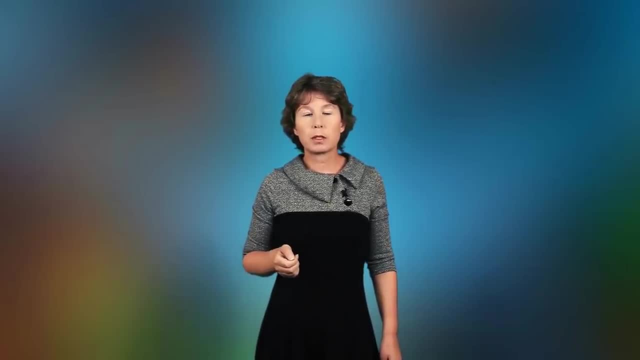 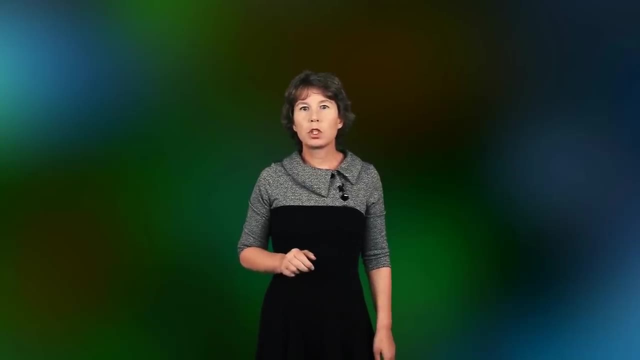 still sent through a classical channel without quantum effects. Quantum Key Distribution is an example for quantum cryptography, But quantum cryptography also more generally refers to using quantum effects to encode messages, not just to exchange keys. But this more general quantum cryptography so far exists only theoretically. 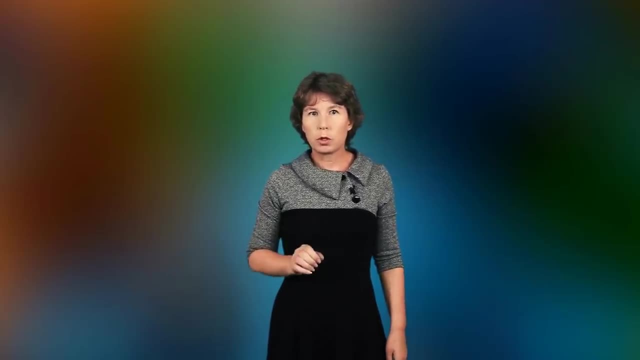 So, to summarize, post-quantum cryptography refers to non-quantum cryptography that cannot be broken with a quantum computer. It exists and it is in the process of becoming widely adopted. Quantum Cryptography is an example for quantum cryptography. Quantum Cryptography is an example. 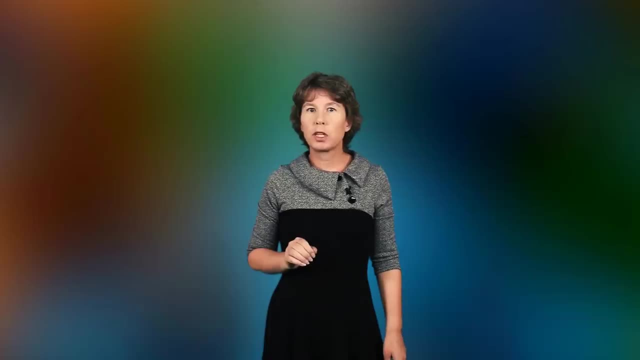 where quantum key distribution exploits quantum effects to share a key that is secure from eavesdropping. It does already exist, though it is not widely used. Quantum cryptography beyond quantum key distribution would use quantum effects to actually share messages. The theory exists, but it has not been realized technologically. 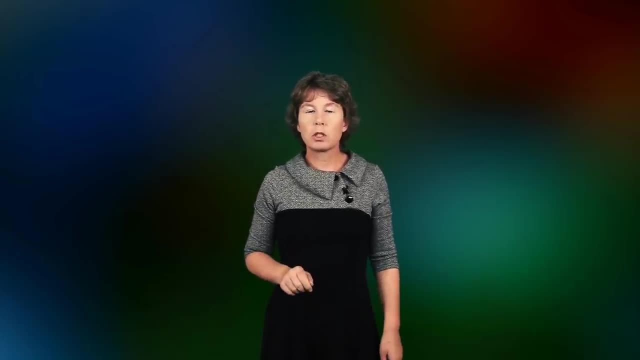 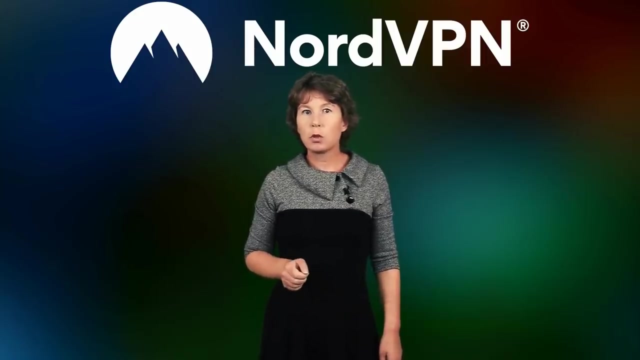 Having said that, let us talk for a moment about your personal security and NordVPN, who have been sponsoring this video. NordVPN is a software that you install on your laptop or phone and it keeps you safe as you browse the internet. It does not rely on a public key system. 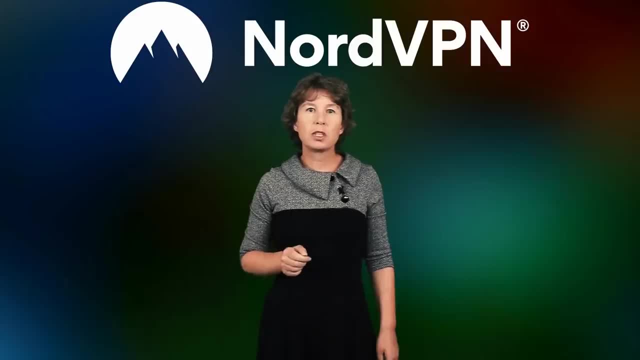 like RSA that I talked about earlier, but instead uses AES. that's the Advanced Encryption Standard. AES is based on a symmetric key that is known to both of the communicating parties. You use the NordVPN app to connect to one of their servers and browse the web from there. This keeps your data. 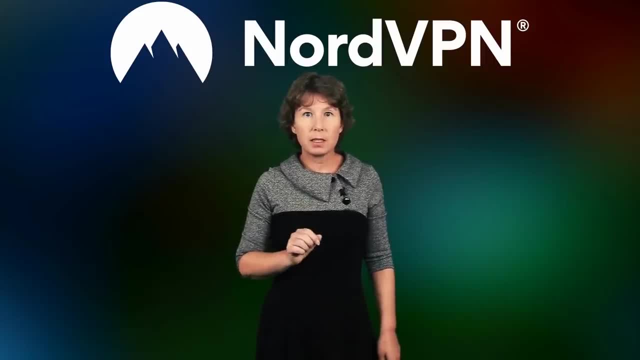 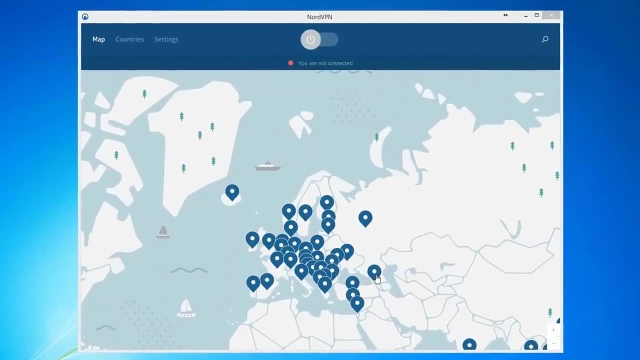 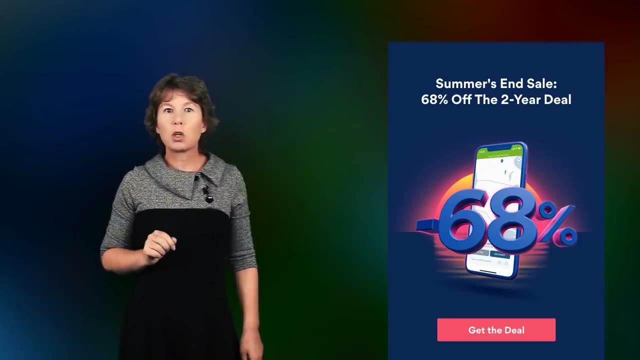 safe, even on a public wireless. Better still, you can choose your location from any one of their more than five thousand servers all over the world. So if you ever encounter a video that won't play where you are, it takes but a click to solve the problem. You can now get sixty-eight percent off. 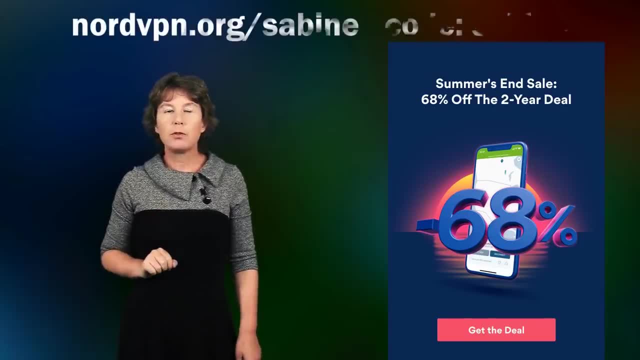 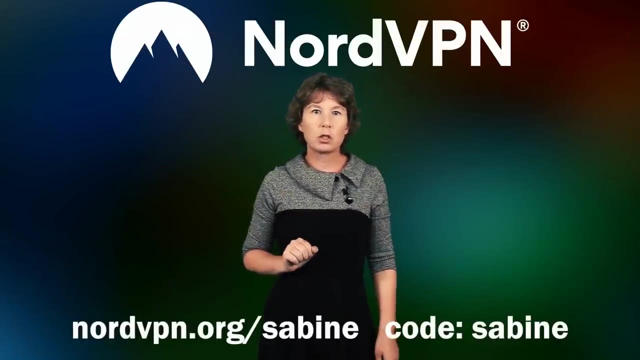 their two-year plan and one additional month free. if you go to nordvpn dot org. slash sabine and use the coupon code sabine, That's S-A-B-I-N-E. NordVPN works on pretty much all platforms: Android, Windows, iOS. what have you? Once again, that's nordvpn dot org. slash sabine. 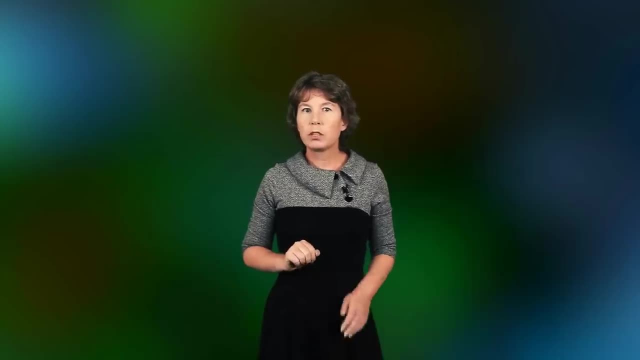 the coupon code sabine. Finally, I want to thank Scott Aronson for fact-checking parts of this transcript, Tim Palmer for trying to fix my broken English, even though it's futile, and all of you for watching. See you next week.